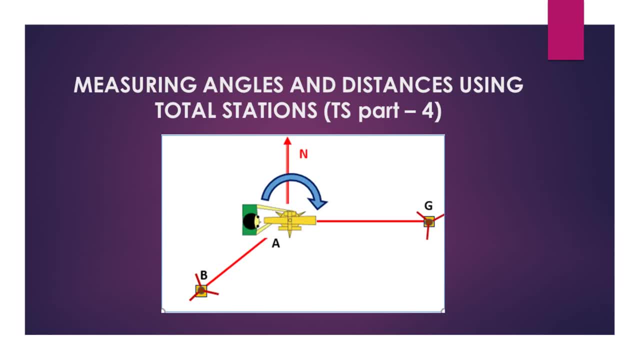 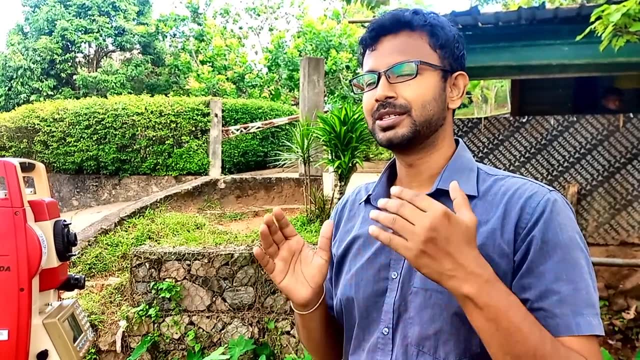 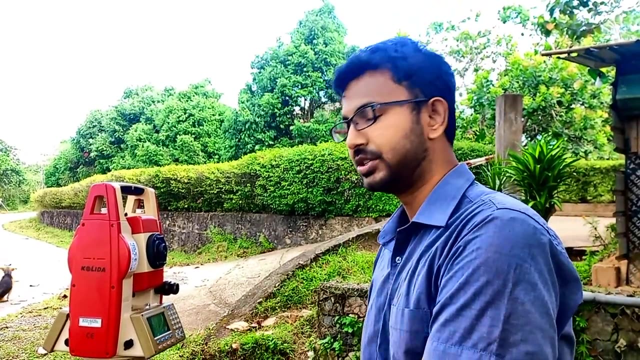 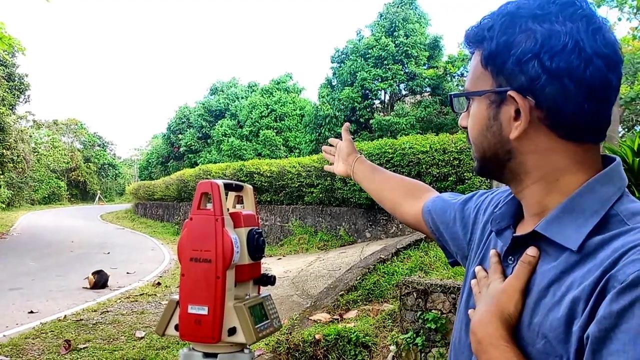 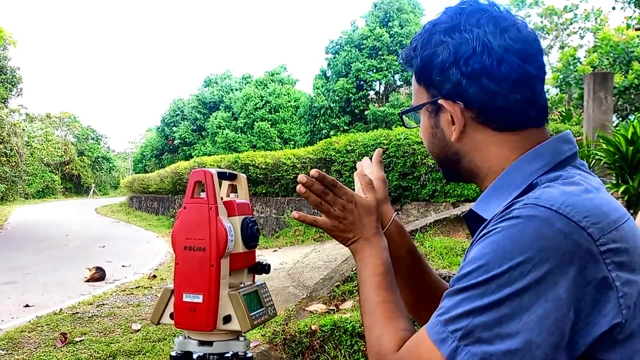 Okay, now we are going to show how to measure an included angle using double phase method. We have set the instrument at 9003 and we are looking at 9002.. This way, we have set up 9004.. So we are going to measure the included angle between 9002 and 9004 from 9003.. 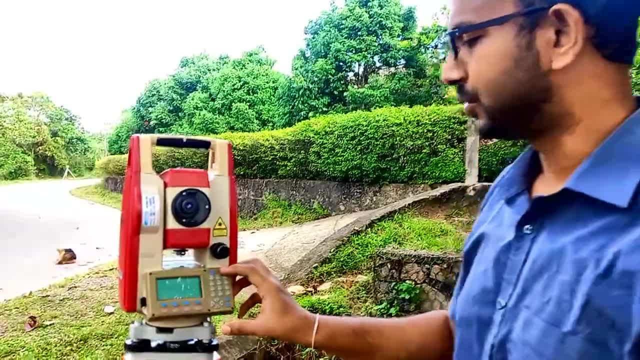 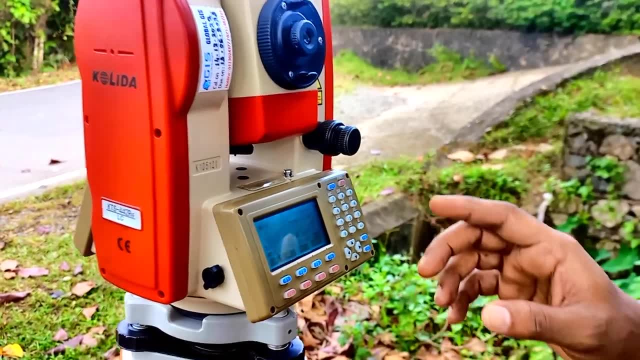 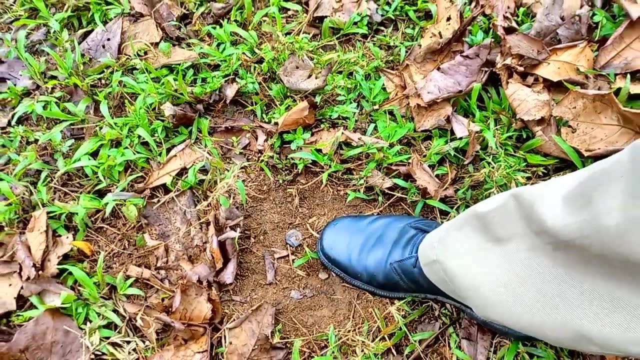 That is what we are going to do. First, we need to switch on the instrument. Soon after we switch on the instrument, I will tell you: first thing is we need to ensure our centering is okay. Now, if you look at the laser point below, you can clearly see it is at the center of the control point. 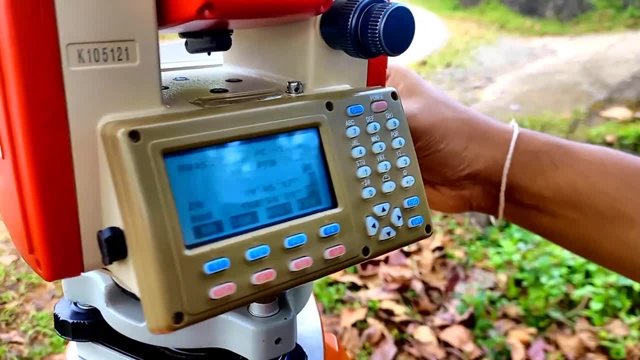 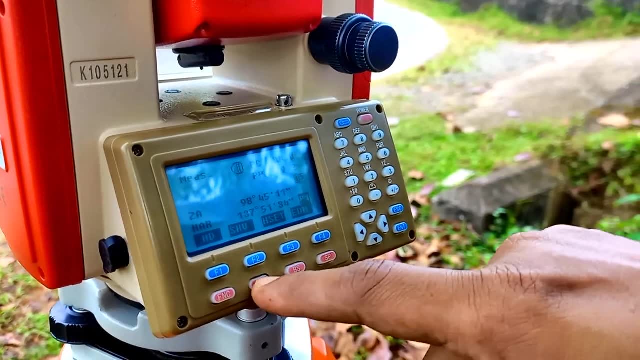 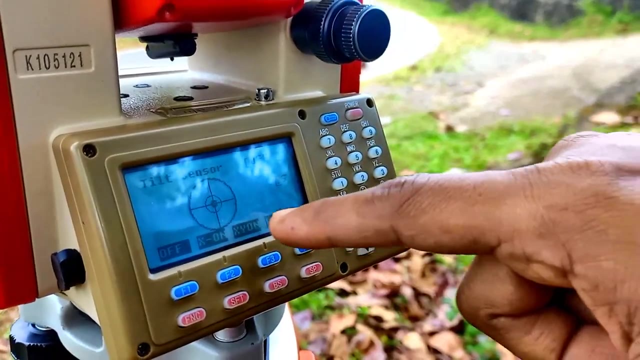 And then we need to check the tilt. First we need to clamp before we press any key. Then we need to press the shift button and go to tilt, Shift and tilt. Then we can check whether the digital bubble is at the center. To me it is okay. 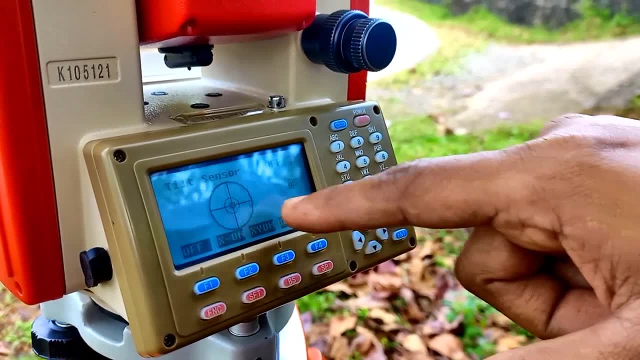 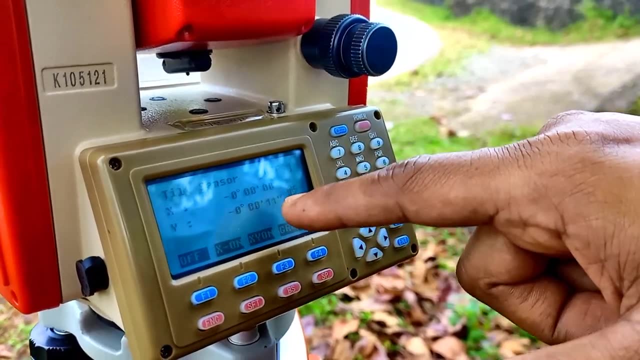 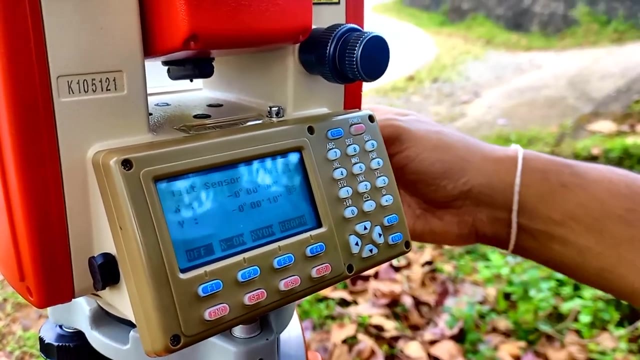 We can check it with the digits. So if we click F4, the button just below the digit, you will get these values. In one direction it is zero. In one direction it is 11 seconds. So we need to bring that 11 seconds to the value less than 10.. 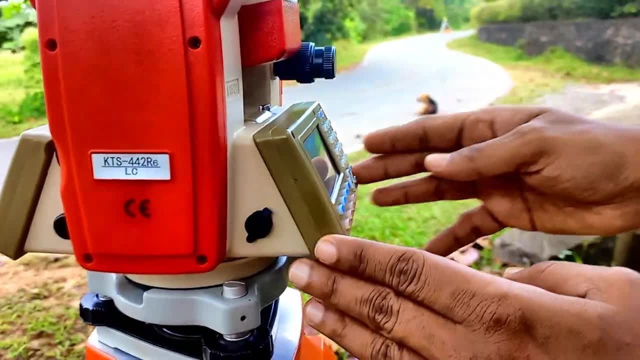 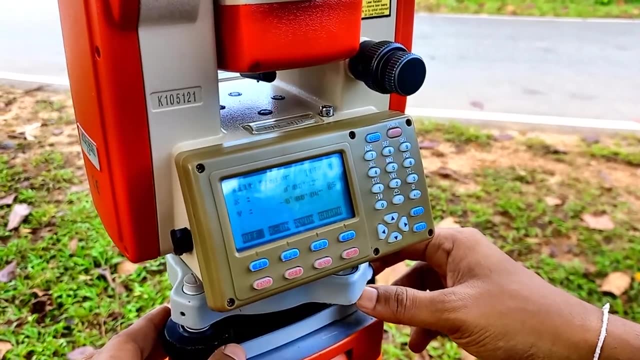 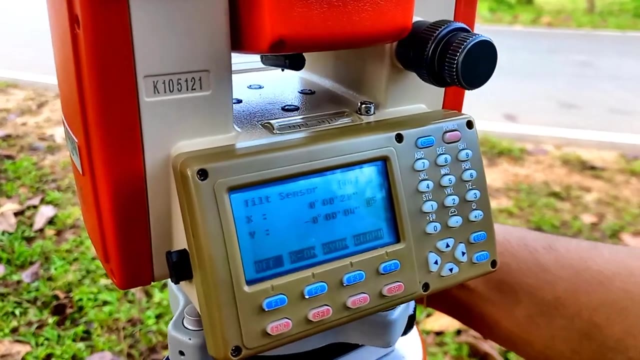 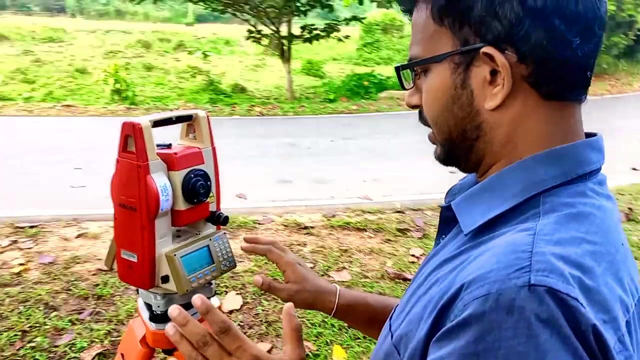 So what I am going to do is I am just keeping this screen parallel to two foot screws like this And try to adjust the bubble. I am using the third screw to adjust this one. Now we have done the centering and leveling. Next thing is we need to check the EDM settings. 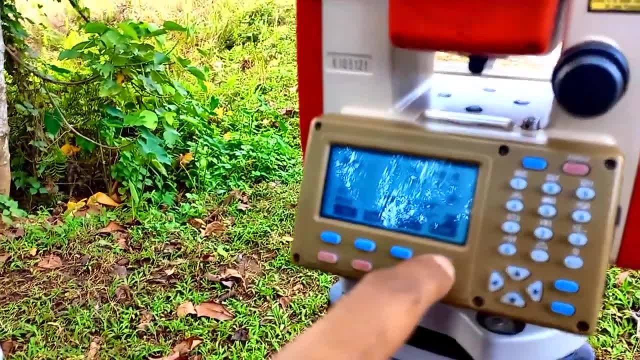 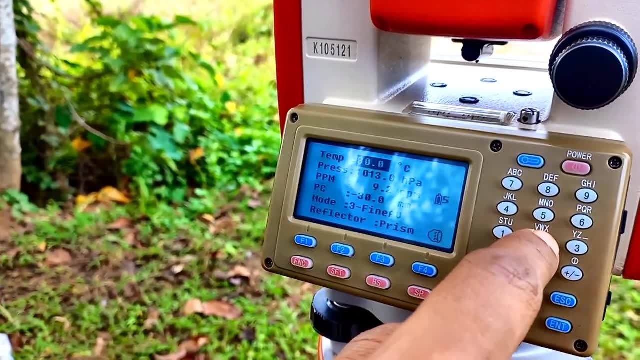 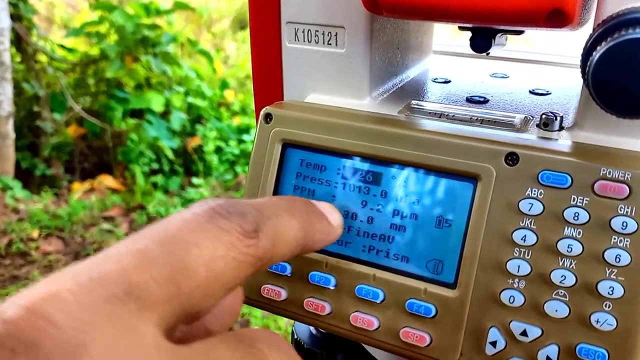 So now we are going to target to the prisms. So if we go to EDM settings, we have the temperature. Now the time is early morning, Therefore we need the temperature is about 26 degrees. When I change the 26 degrees you can see the PPM value will change automatically. 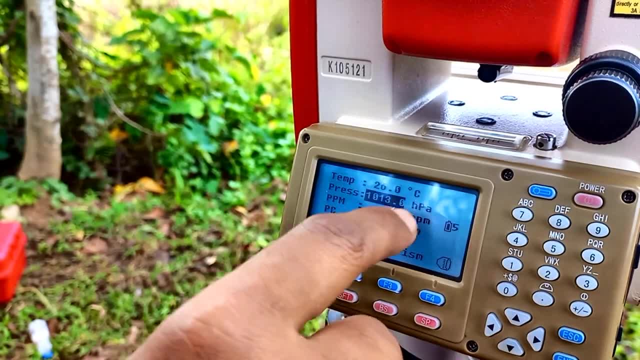 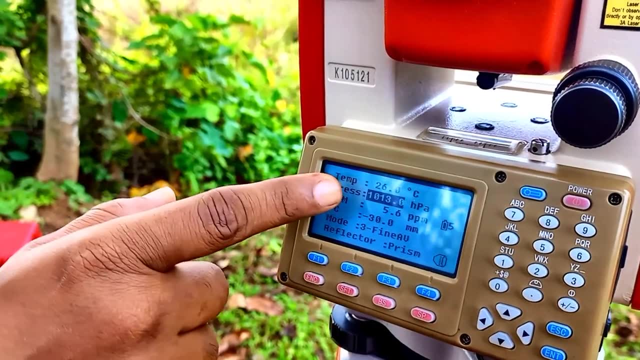 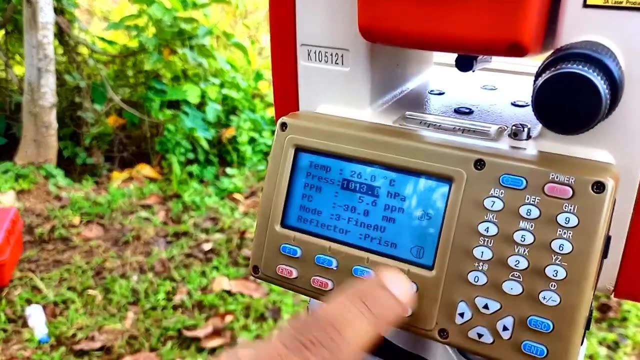 It has become 5.6.. PPM: that will adjust automatically. The pressure is okay because it is the atmospheric pressure, 1013 at the mean zero level. So prism constant is minus 30. So we are not going to change it. 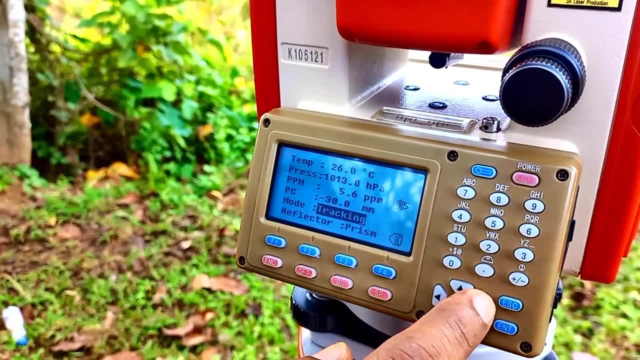 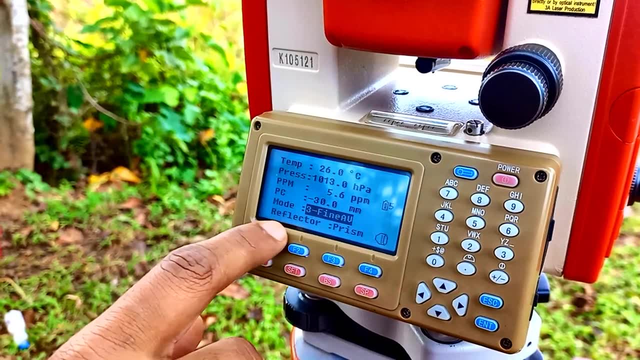 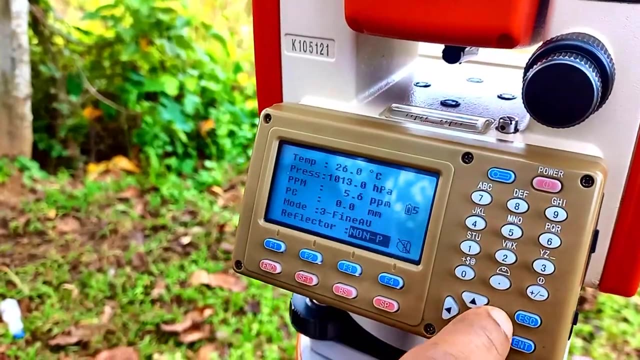 And the mode is fine average. So there are several modes: fine hour tracking, So fine, average will give you the average value after getting three readings. So reflector is prism. So if we change it, you see, if we make it non prism, the prism constant will become zero. 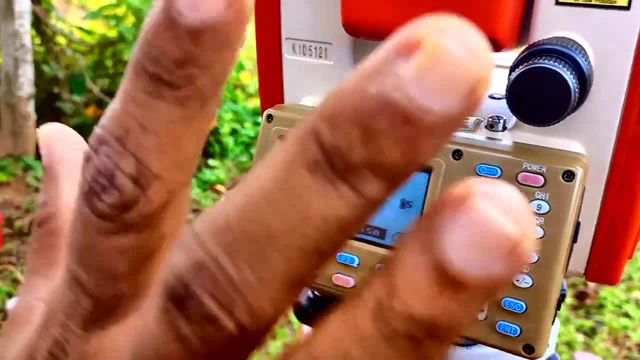 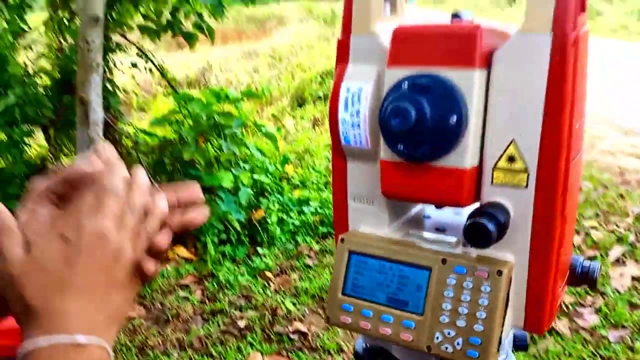 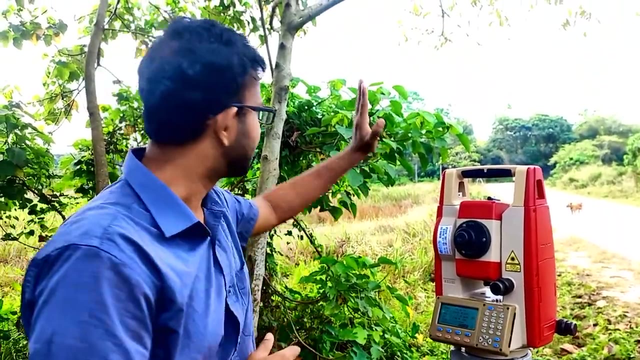 Sheet, again zero, But prism it is minus 30. So after adjusting all these settings, then only we are going to measure the angles and find the distances. So in any traverse we need to measure angles and distances. So now we are going to measure the included angle from the 9002 point to 9003.. 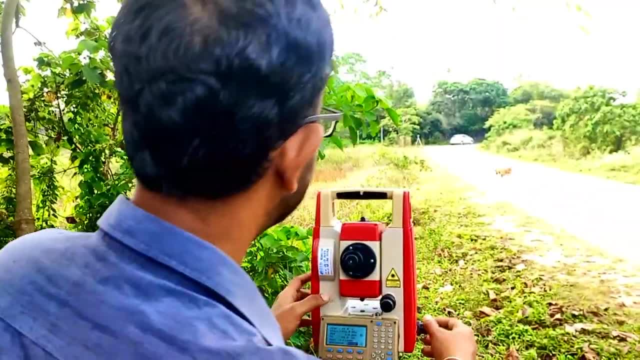 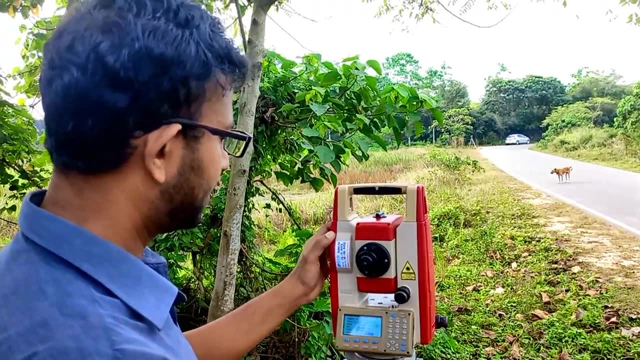 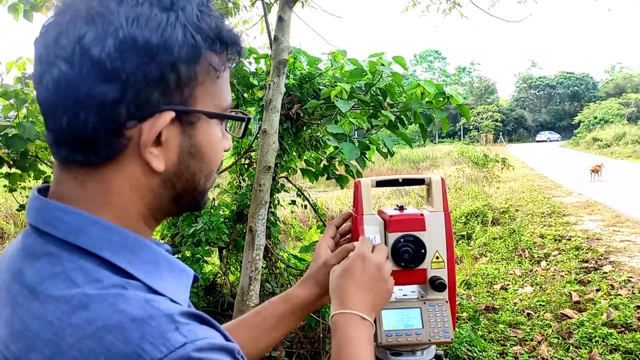 So first I am going to target the total station to 9002.. So first I want to make the instrument into the face left operation. So now it is in the face left operation, The bigger part of the handle. So this is the carrying handle. 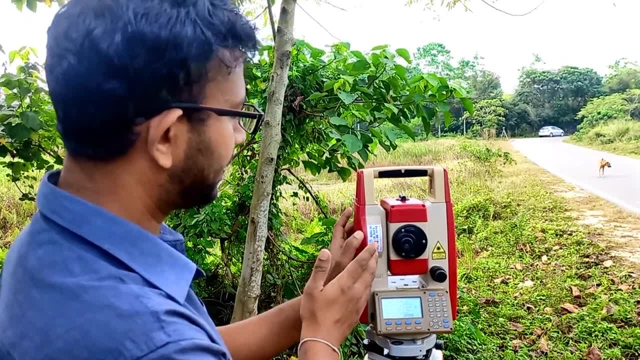 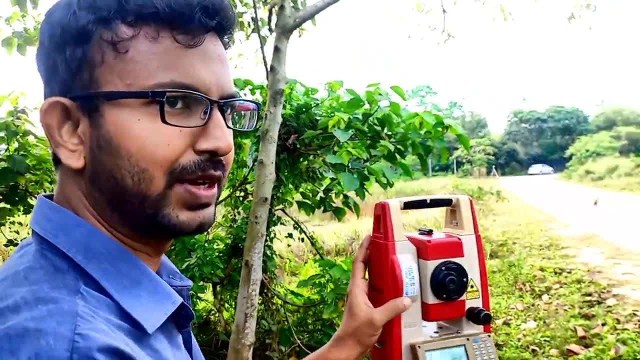 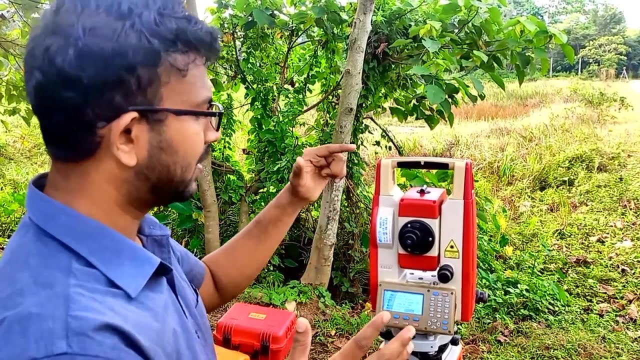 So this part of the left side part of the instrument should be bigger than the right hand side. So that's how we identify it. We identify it as face left, Right. So face left And that has come from the older instruments. In the older instruments the vernier scale was there in the left hand side. 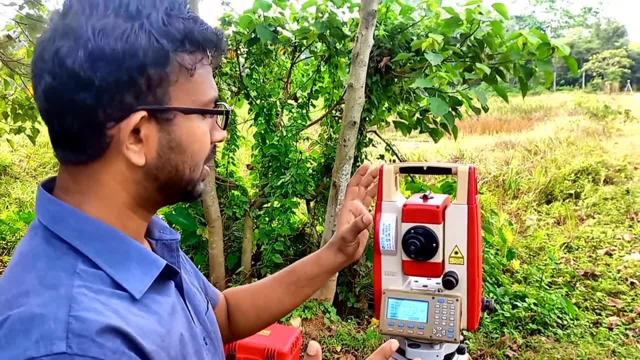 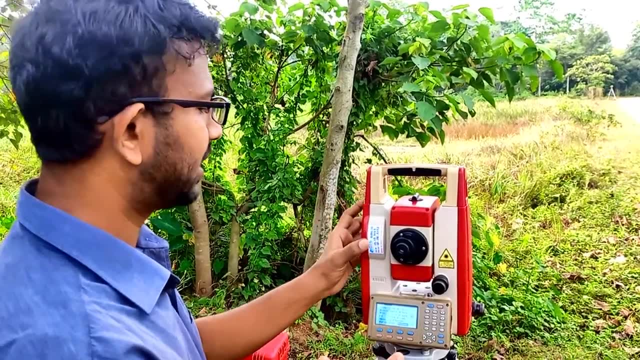 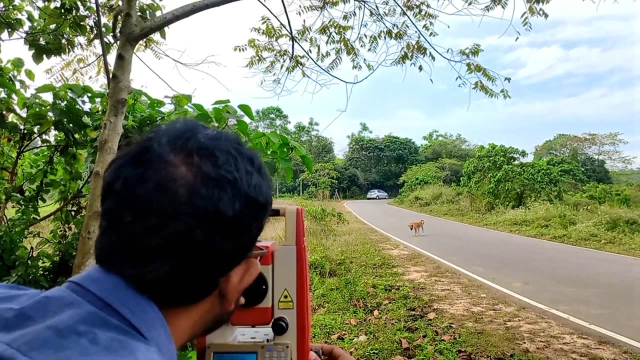 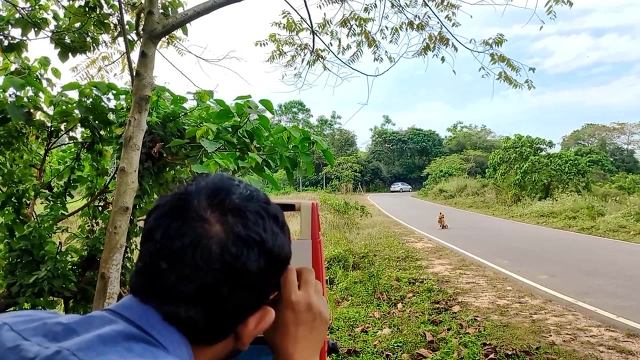 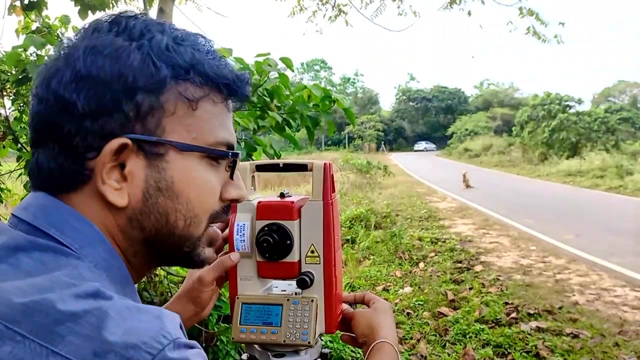 To resemble that the left hand side of the instrument has been made bigger than the other side To accommodate all the electronic parts in the left hand side, Right. So now we are going to target to 9002.. Right, So this is how I target. 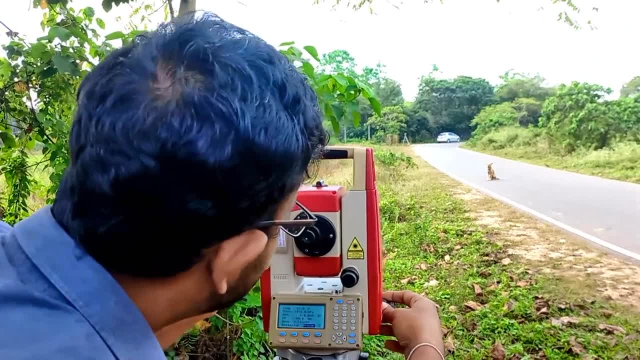 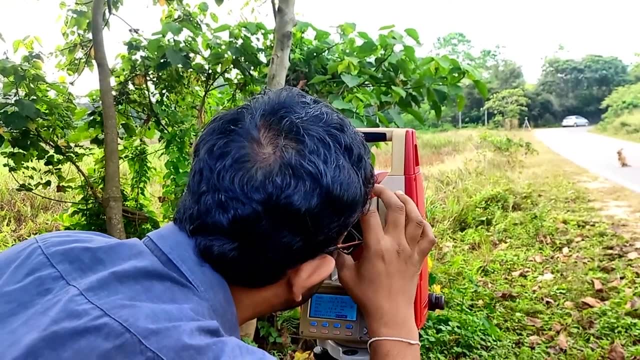 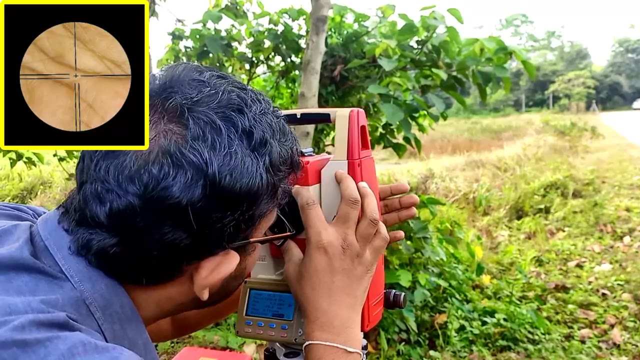 First I need to see through the gun sight And target to the head of the piston And then clamp, Then focus the procea focusing screw Right And I clear the procea focusing screw And then I clear the object focusing screw. 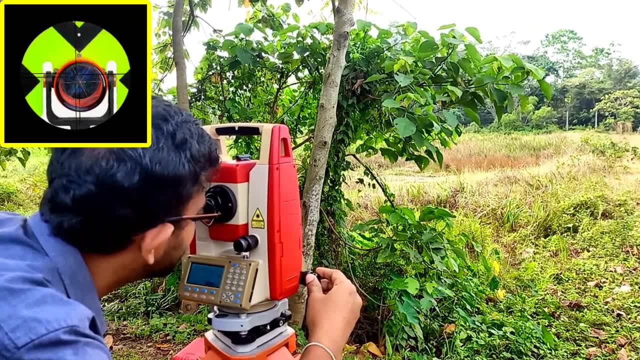 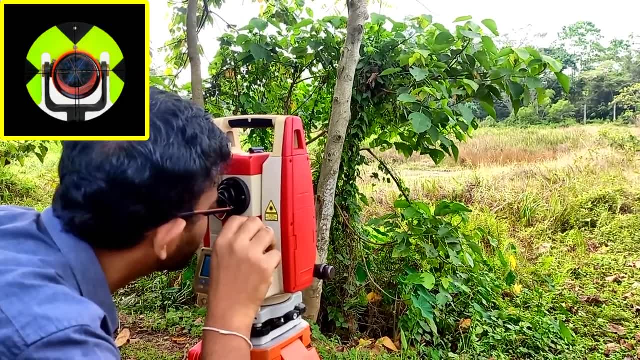 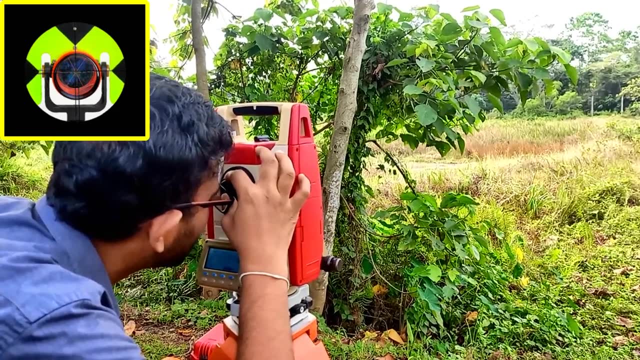 Then I target to the prism Right. In my last videos I have explained how to target to the prism Right. Now I have targeted to the prism. The procea should cut the down head arrow and the side arrows of the target prism bolt. 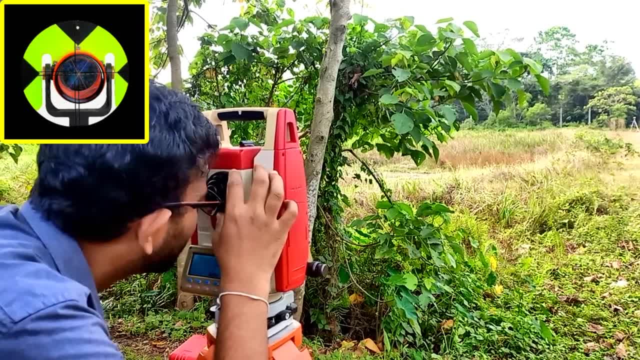 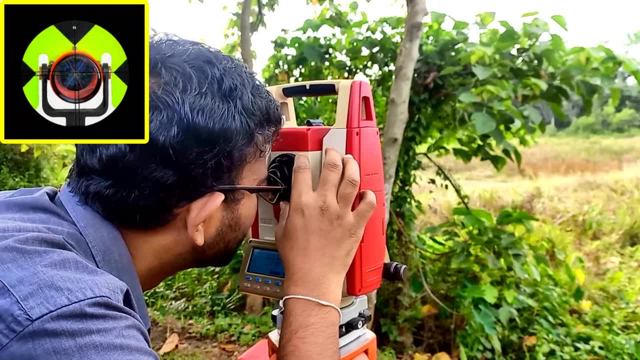 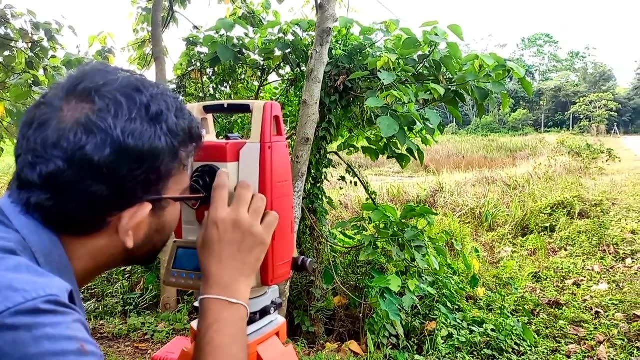 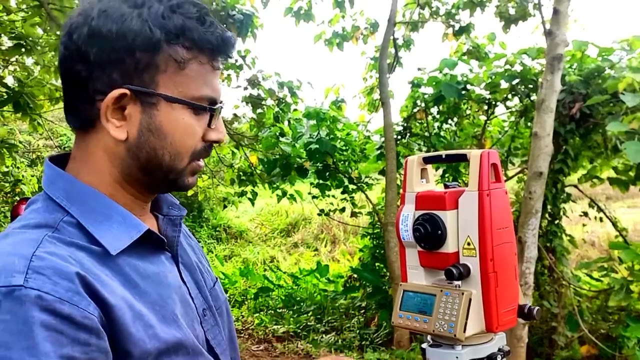 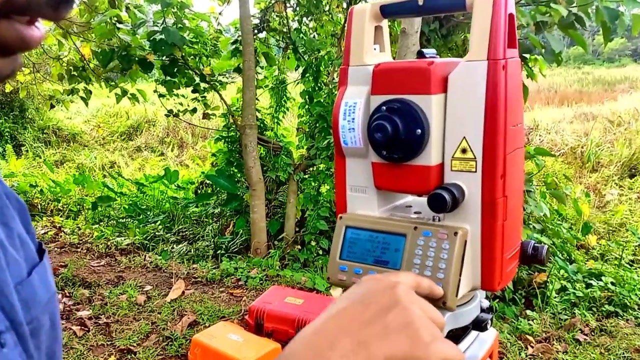 I need to move my eye side by side until the procea has no relative movement. With my movement of the eye Right Now I have targeted exactly to the prism. So now I have to escape from this page- Right Escape. Now I need to go to H-set. 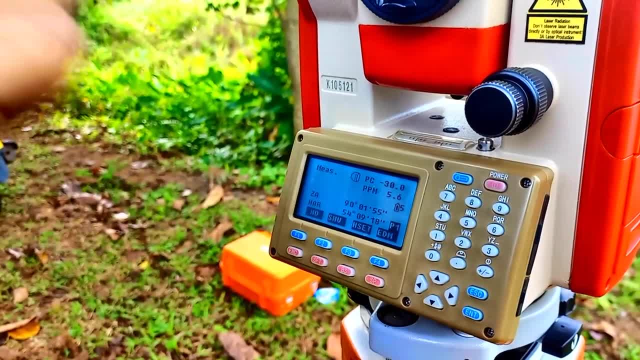 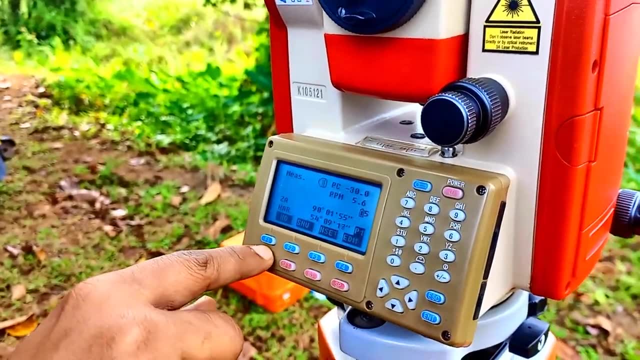 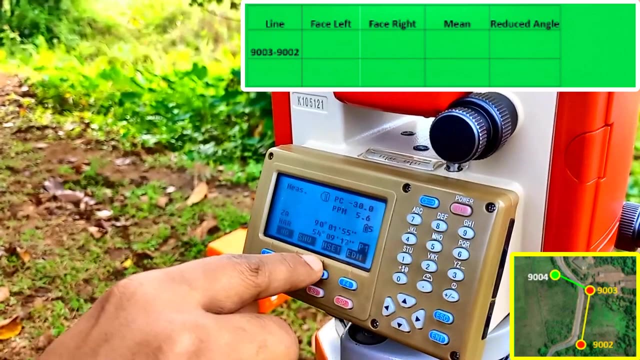 H-set is the button that I should press to give a desired angle Right. So if you do not find H-set, then you can go to this function and see whether H-set is there Right. So I press the function Now. I find H-set here. 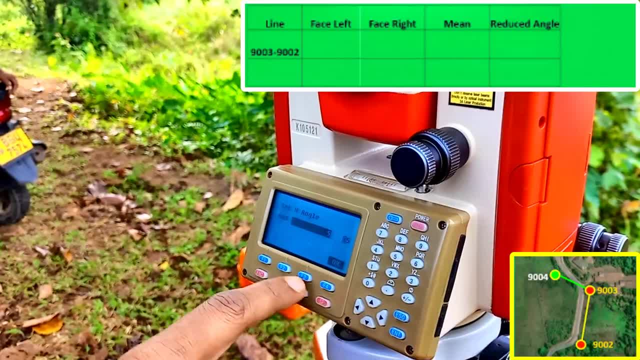 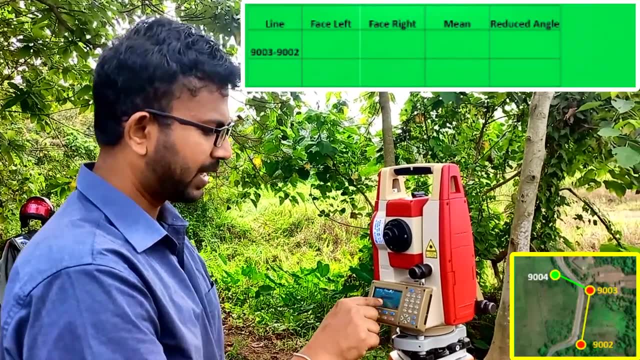 Right, I prefer to set 5 degrees here, Right, Because if we set 0 when we are doing the calculation it is very difficult, Right? So therefore I press, I set 5. 5 to that angle. Right, I set 5 and click OK. 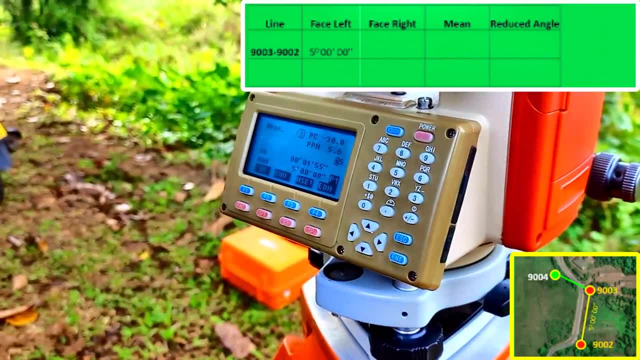 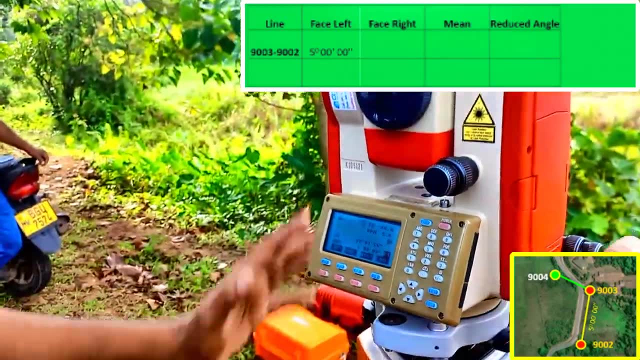 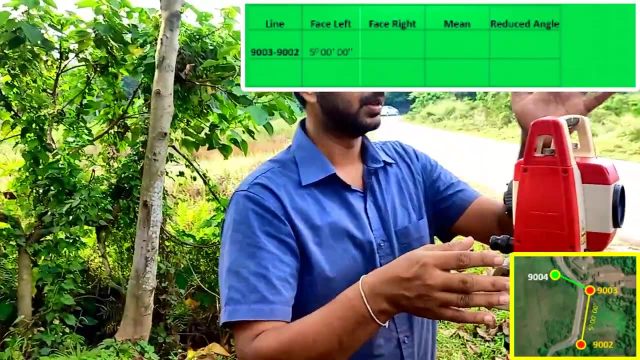 Now you see the HAR has become 5.. That is the horizontal angle I have set to that 9002 target Right. So now I am in the face left operation. So I am now going to turn it and target to the prism. 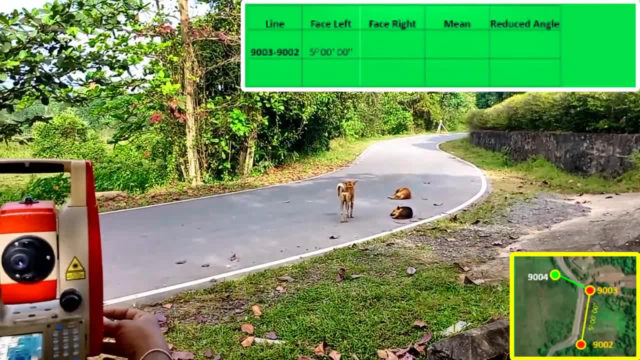 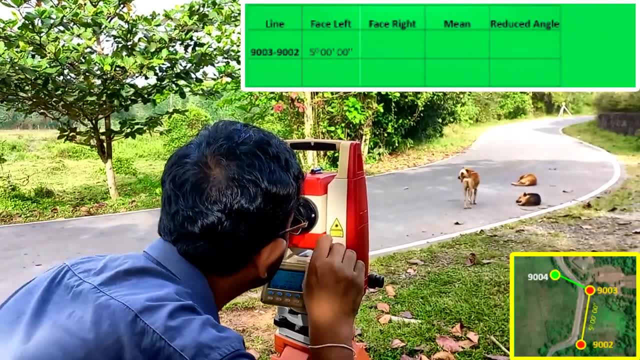 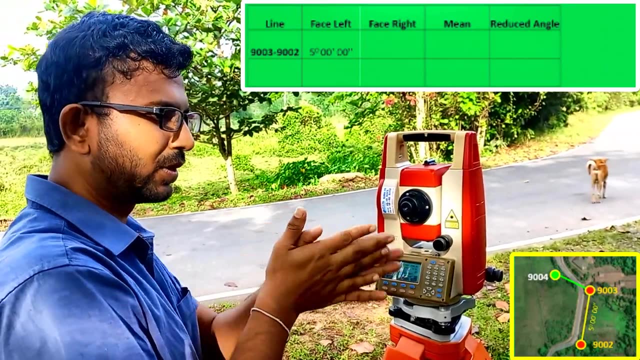 So now I am going, I am going to turn it and target it to the 9004 prism Right When I am turning the instrument. I need to turn it clockwise So you can turn it anti-clockwise as well. Then you will better understand that we are taking the clockwise angles. 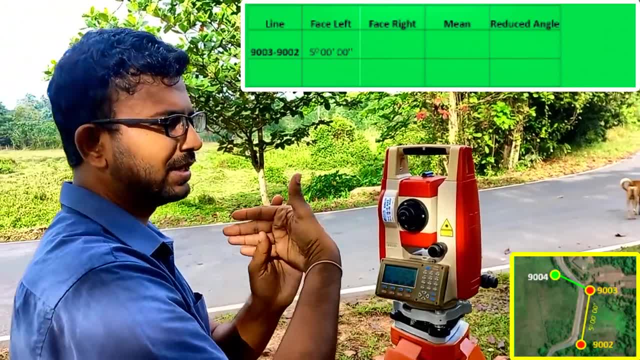 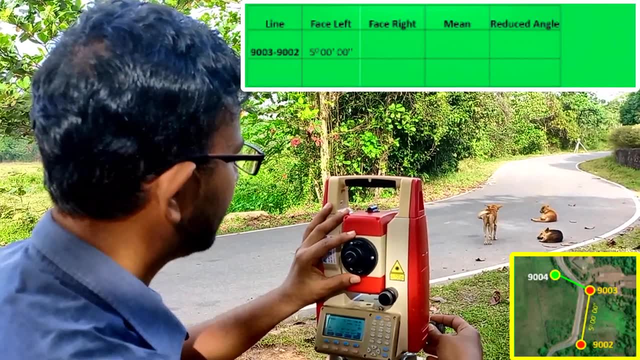 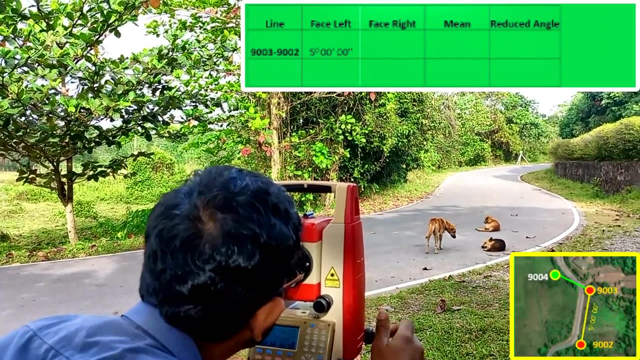 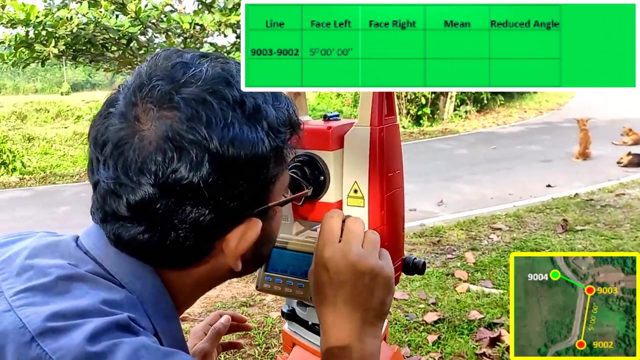 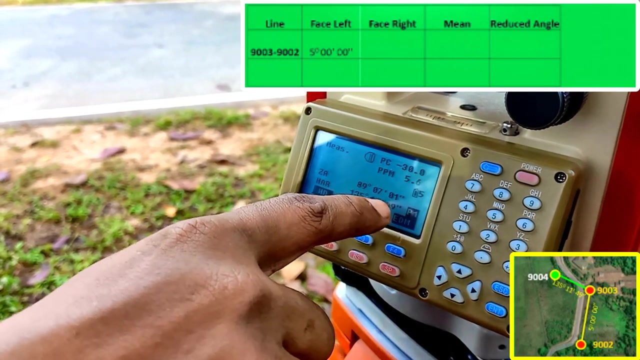 Right. That is why it is better to turn clockwise, because the included angle is clockwise angle between two legs. That is why we turn the instrument clockwise to get the reading of next control point Right. So now the value is 135,, 11,, 49.. 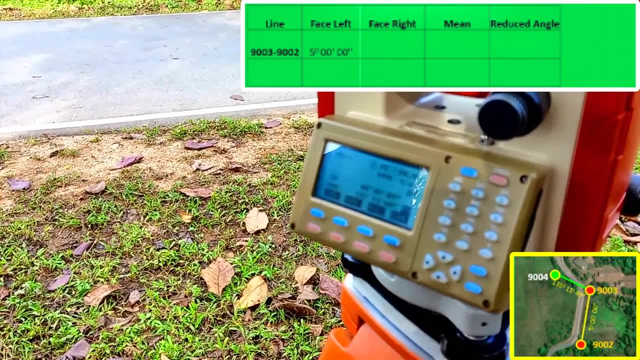 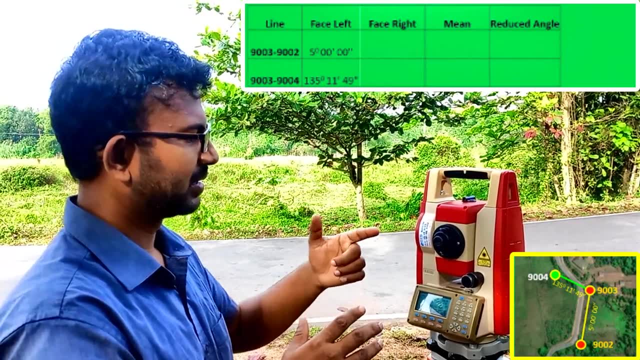 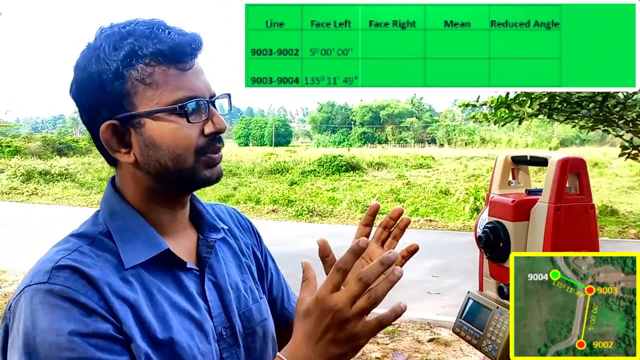 Right: 135,, 11,, 49 is the value. So that is the face left reading Right To remove the instrumental errors. just like the telescope axis is not exactly perpendicular to the funion axis, like that errors, we need to get the face right reading as well. 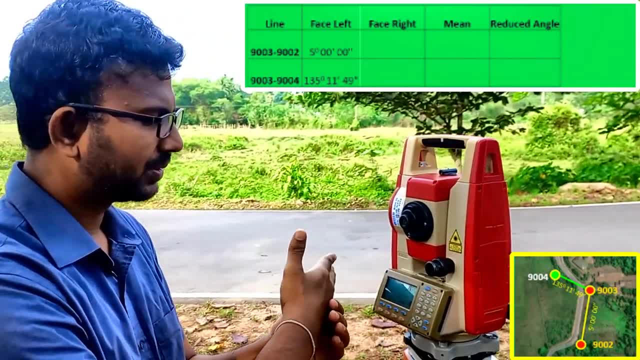 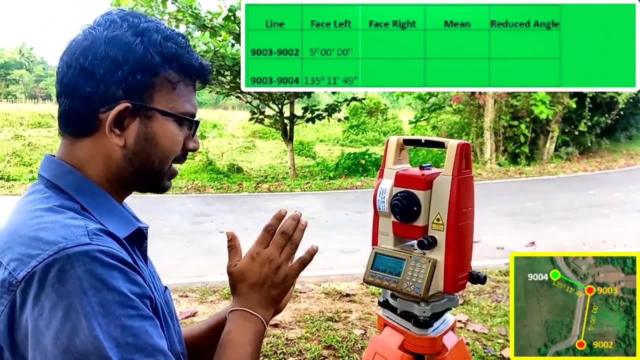 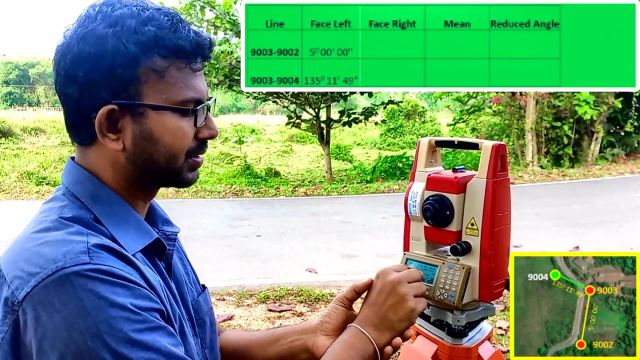 Right To the same targets. Now, when we are turning the instrument, only the upper part is turning and the lower part is as it is there. Right, When the upper part or upper plate of the total station turns, the reading increases. Right Now, without turning the upper part, we are going to transit the telescope about the funion axis. 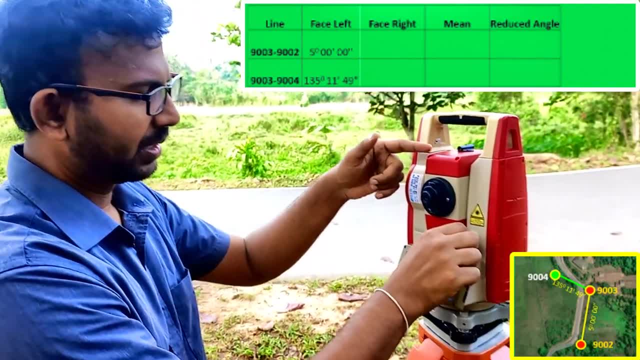 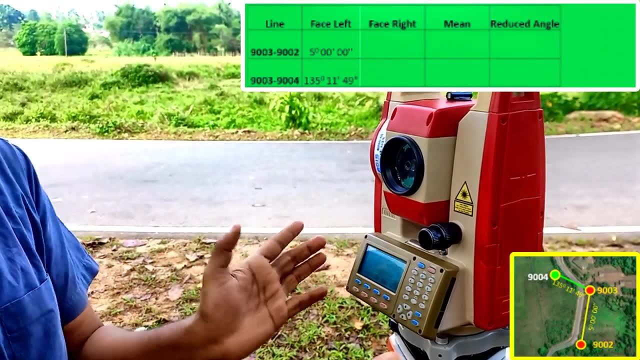 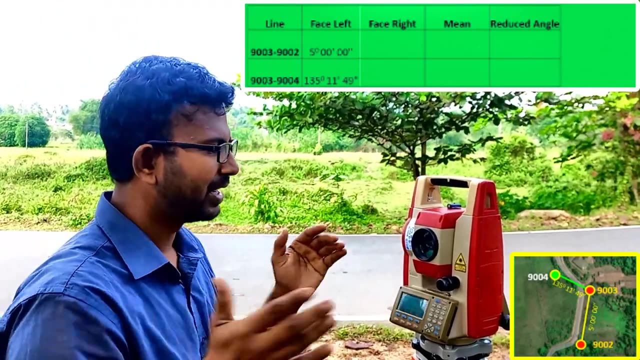 This axis is called funion axis. I unclamp clamping screw. I unclamp the vertical clamping screw and transit Transit without turning the base plate. Right Now I have cheated the instrument. Right Now. instrument does not know that I have turned it 180 degrees from the direction where it. 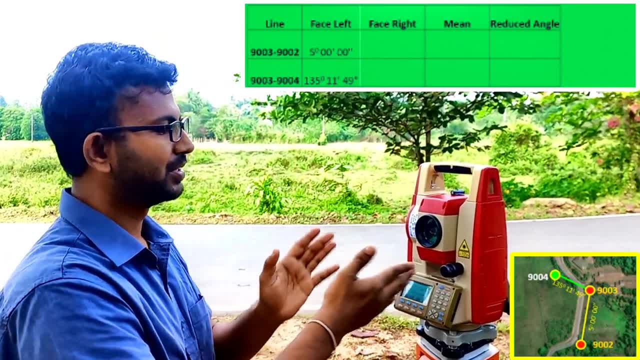 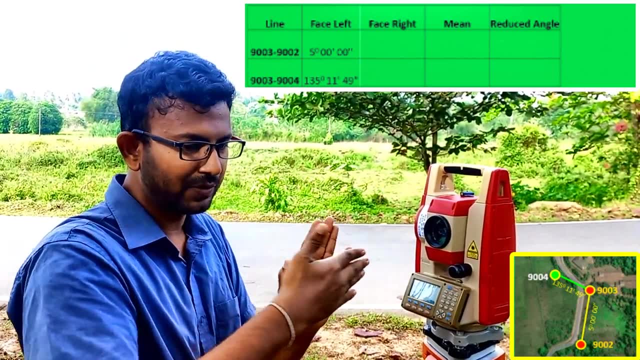 was looking previously. Right, So now I am going to target back to the 9400.. Right. Then, when I am targeting back to the 9400, I need to turn the instrument about 180 degrees Right, Exactly 180 degrees. 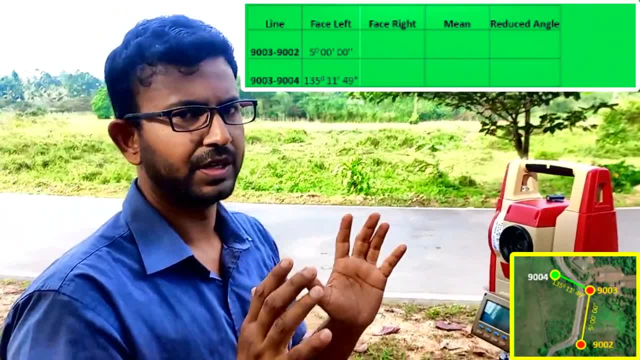 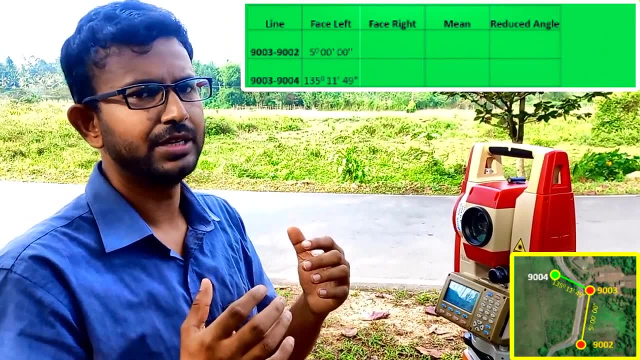 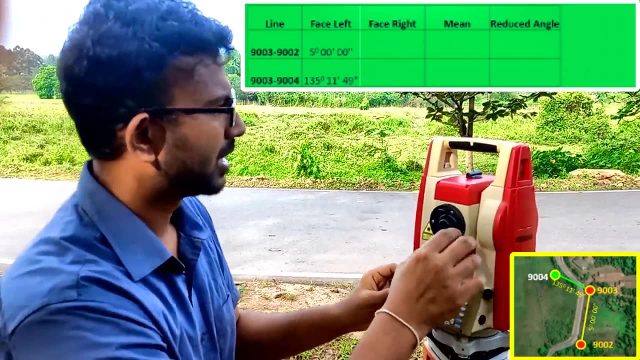 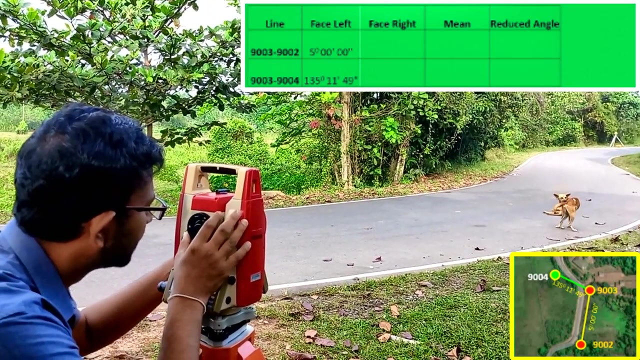 If the instrument has made perfectly, the difference between the face left reading and the face right reading should be exactly 180.. Now we will see what is happening. Right, So now I am going to turn it and target back to the 9400.. 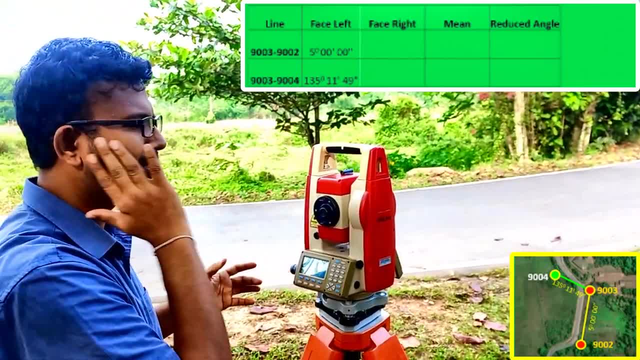 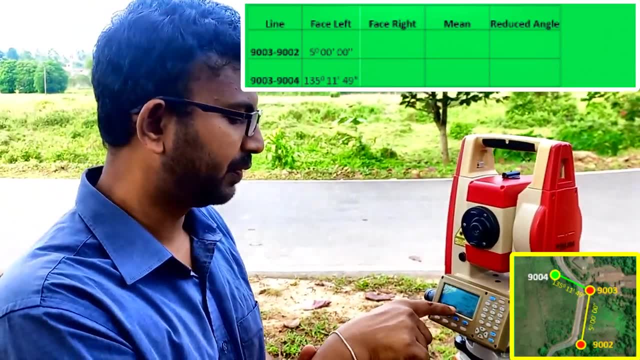 Now you see, the bigger part of the instrument is at the right hand side of my face, So it is face right operation. Now you see the face right reading is 315, 11 minutes and 44 seconds Right, So it should be 315, 11, and 49.. 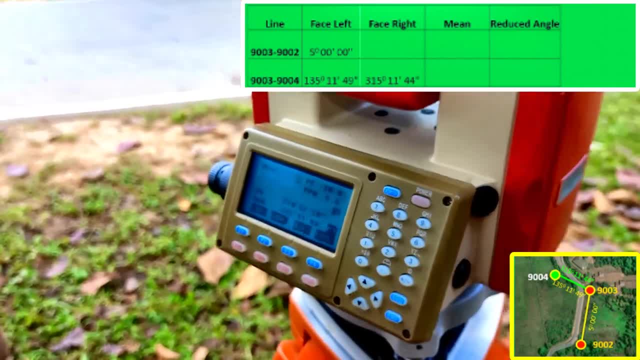 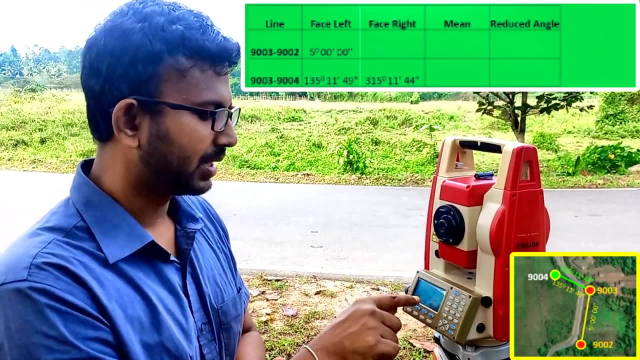 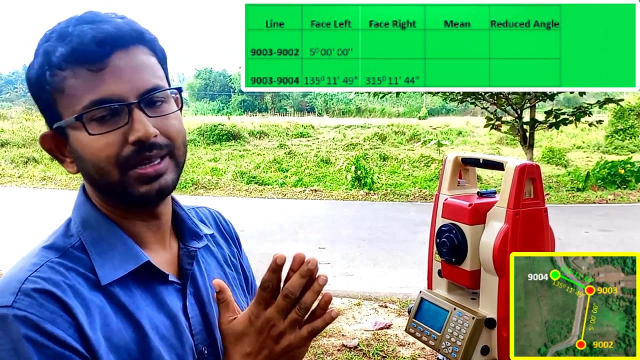 Right, But the value is 315,, 11, and 44. Right, That means the instrument is not made perfectly Right. Some instrumental errors are there, Right, So we need to record this angle. face right angle to the 9004 as well. 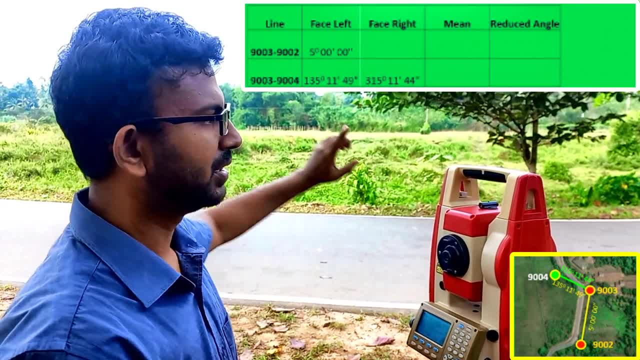 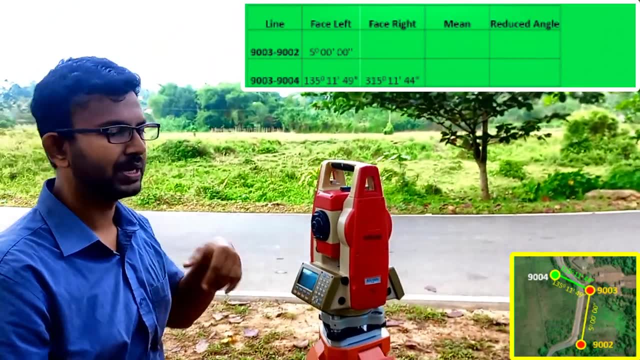 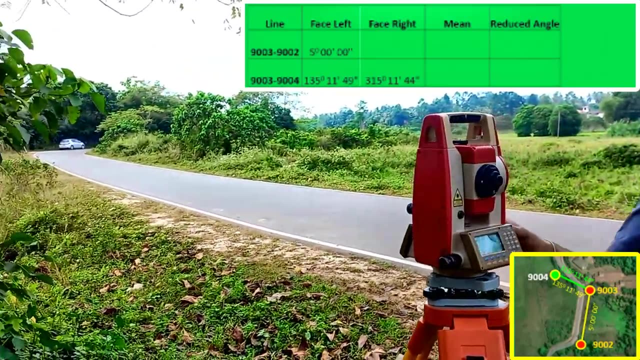 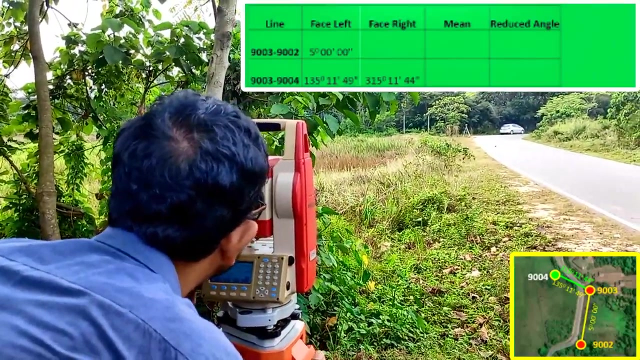 The next step is we are going to take the face right reading to the 9002 as well, thousand two as well. that is the first uh point where we targeted from the facelift right. so we are getting it at last. right now, you see, the reading is 184 59. 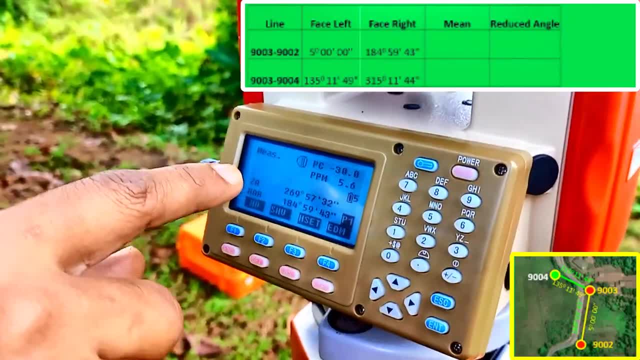 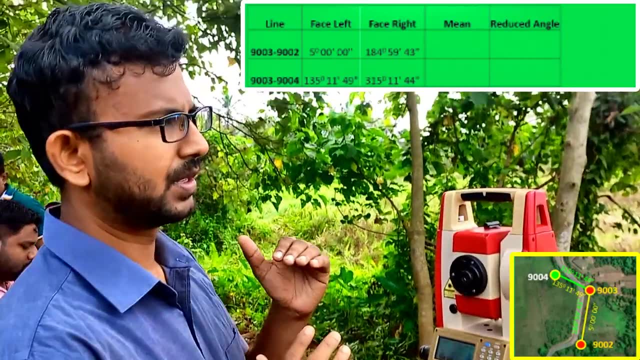 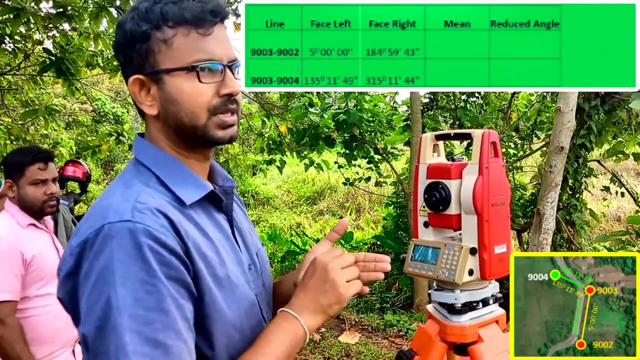 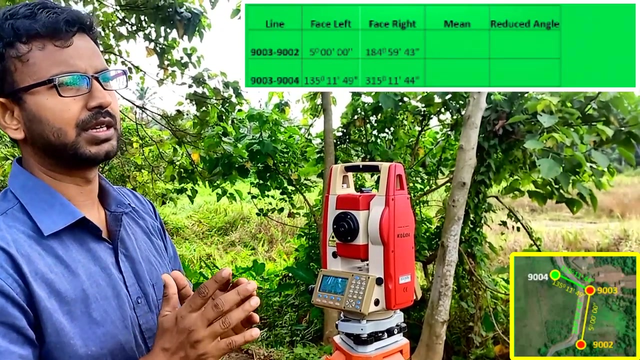 49, 43. it should be 185, right, but the value is 184, 59, 43, right. that means uh, again we it. we confirm that there is an error in the instrument, so we need to record this face right reading to 9002 as well. right now we can get the mean of this: facelift and face right. 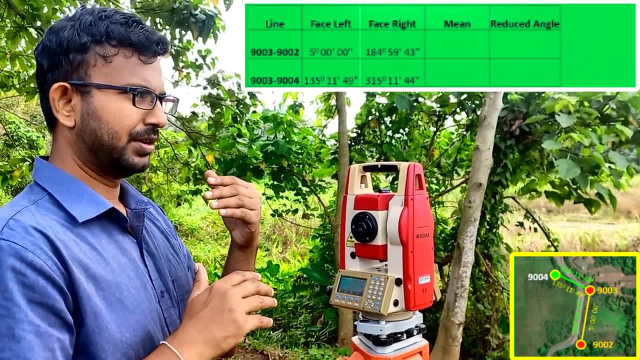 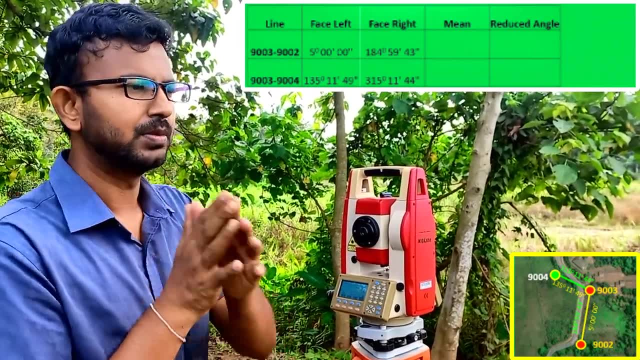 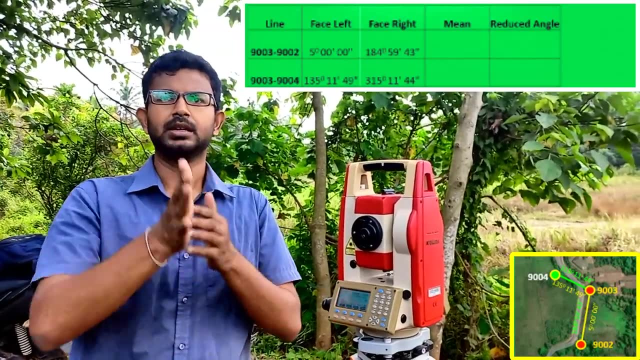 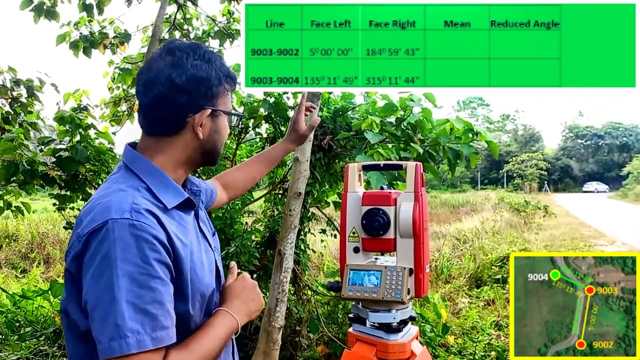 readings and obtain the reduced angle for the included angle between this 9002 and 9004, measured from 9003 right. so next step is we need to find the distance distance from 9003 to 9004. since this is a control line, we don't need to. 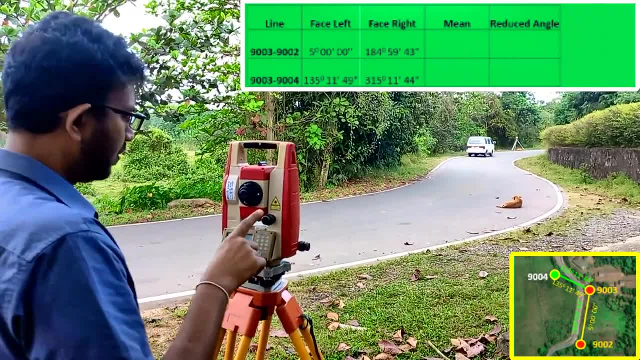 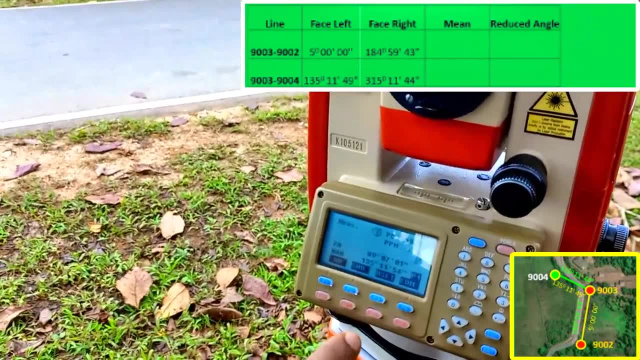 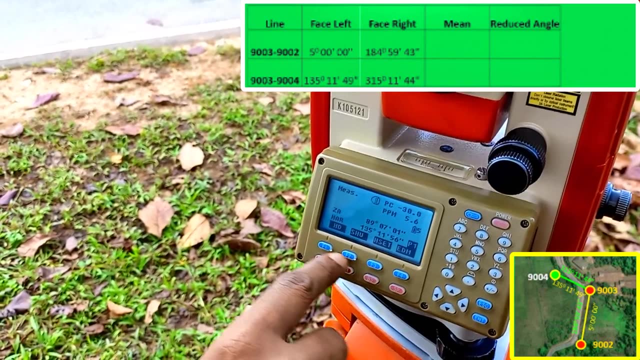 find the distance in this line. now i need to find the horizontal distance right: horizontal distance from 9003 to 9004. for that again i need to find out the suitable option from the key pair right. so here in the display it shows hd shv. 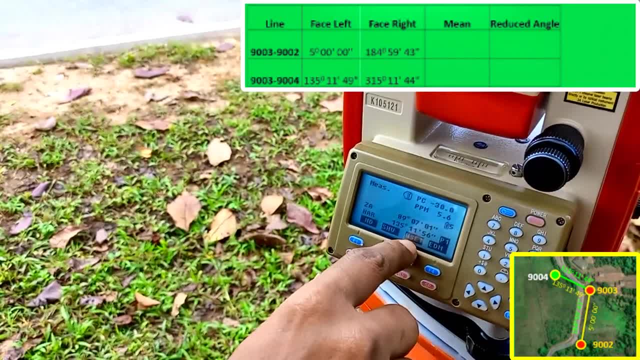 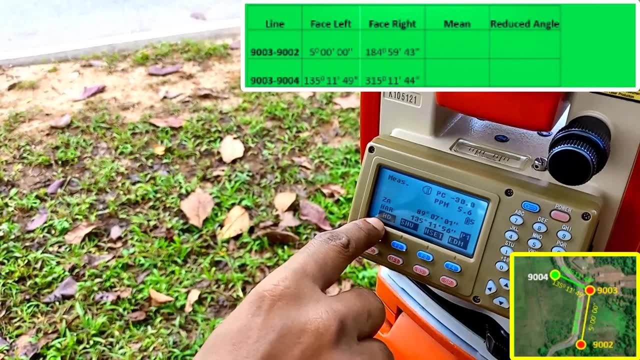 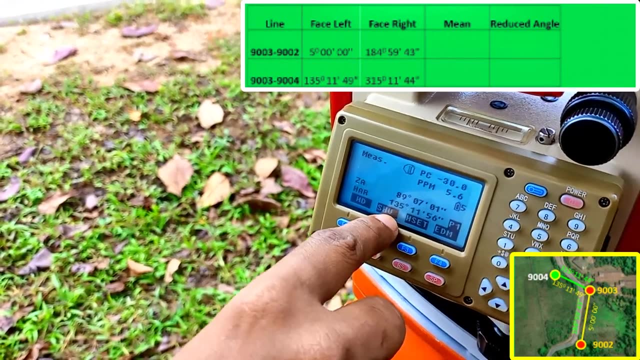 horizon, hset, edm. hset was the one we were using early right, so now we need to find out the horizontal distance. for that. hd is the option right. hd means horizontal distance. if we press shv, shv will give you the slope distance, horizontal distance and vertical difference. 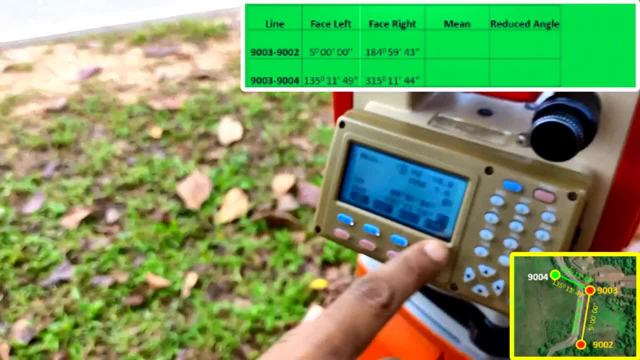 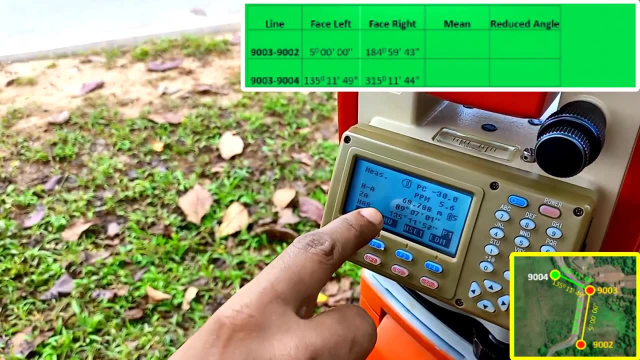 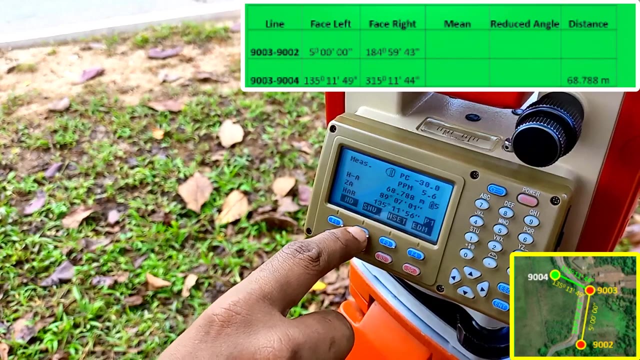 from this point to that control point, right. so now i'm going to press hd. when i press hd now you see three readings were taken and the average distance is displayed here it is 68.788. now if you click shv you will see. now this is va. va is the vertical difference between the prism. 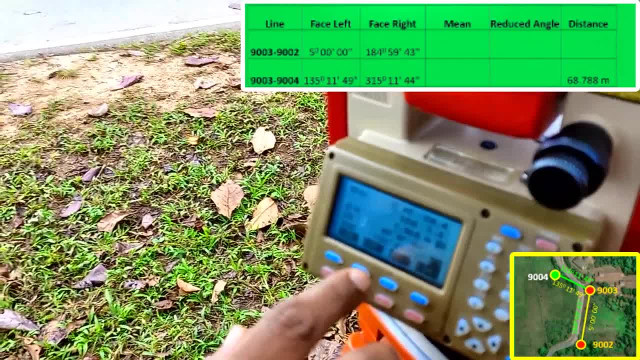 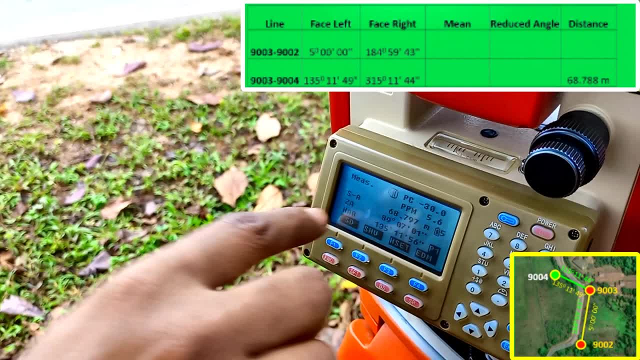 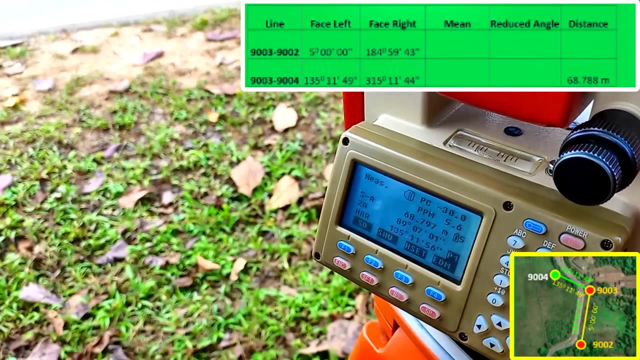 and this total station telescope right. and then, if i press again shv, you will get the slope slope distance. it is 68.797. it is greater than the horizontal distance right. always the slope angle or the slope distance is greater than the horizontal distance right. if we 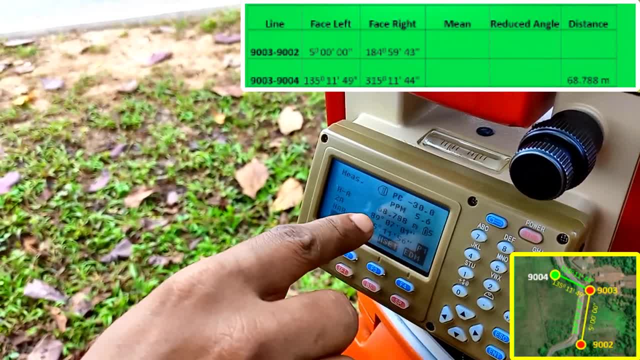 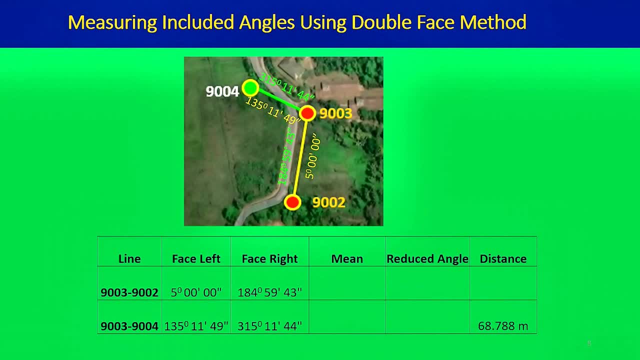 click shv, it is 68.797. it is greater than the horizontal distance right, always the slope angle. press back shv ha, the horizontal distance will give back 68.788. that's how you find out the horizontal distance using the total station. now we'll see how to get the mean values of face left. 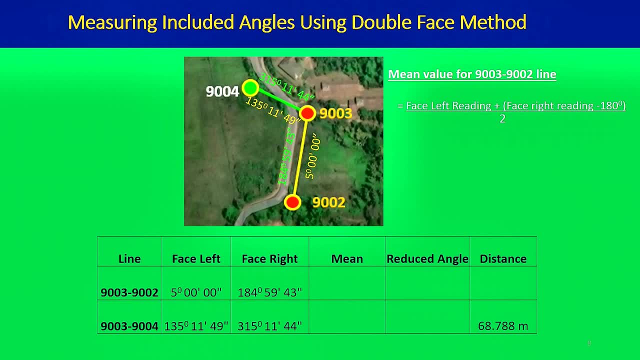 and face right reading. first of all, what we need to do is we need to deduct 180 degrees from face right reading to correct it. after that we have to add it to the face left reading and divide it by two to get the mean value. then we have to add four degrees, 59 minutes and 43 seconds to 5 degrees and divide it by 2. 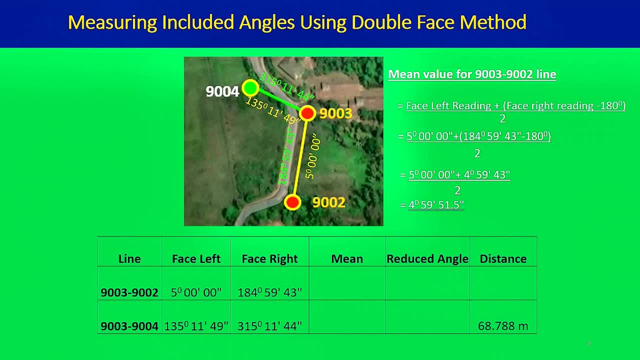 then the mean value is 4 degrees 59 minutes 51.5 seconds, so we can record it in the mean column. similarly we can find the mean value for 9003, 9004 line. again we need to deduct 180 degrees from face right reading to correct it and then add it to the face left reading and divide it by two. 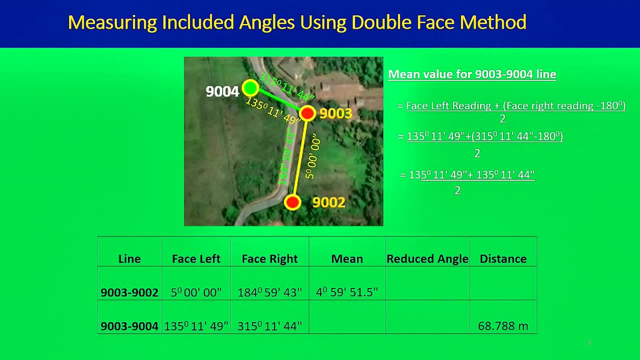 then we need to add 135 degrees, 11 minutes and 49 seconds to 135 degrees, 11 minutes and 44 seconds and divide it by two. then the mean value is 135 degrees, 11 minutes and 46.5 seconds and we have 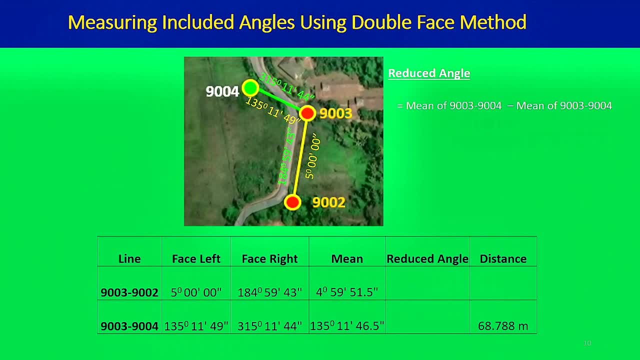 recorded in the mean column and then we need to find out the reduced angle. for that we need to deduct the mean of 9003 9004 line from mean of 9003 9004 line. then The deducted radius angle is 130 degrees, 11 minutes and 55 seconds. So that is how we find. 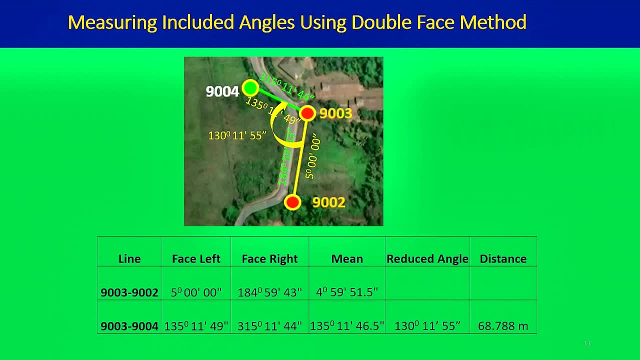 the radius angle or the included angle between two points or two stations from the station where the instrument operates. Similarly, we can carry out the traverse using angle and distances. So today we learn how to measure an included angle. not only that, but also how to measure a distance.